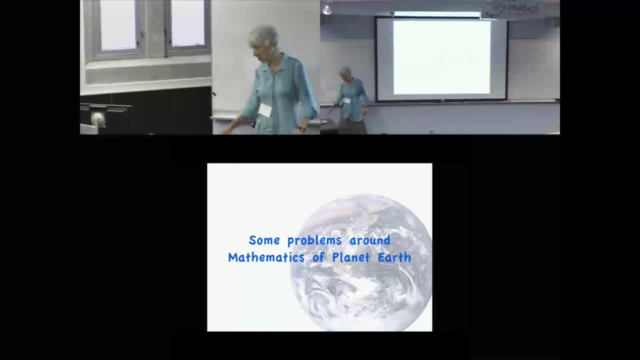 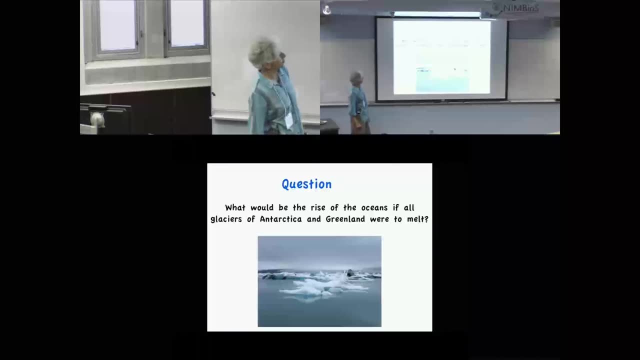 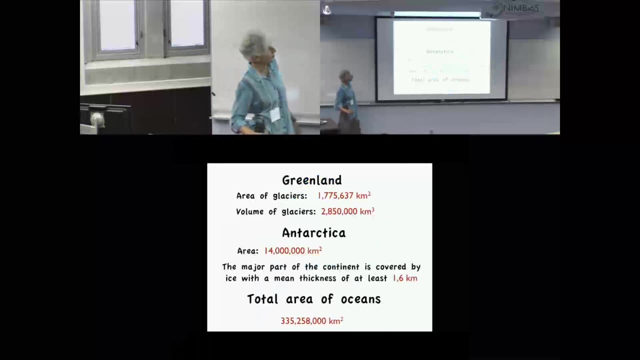 I will go with examples, In fact, examples sometimes that you can do in your classroom. For instance, a question: What would be the rise of the oceans If all glaciers are gone? what would be the rise of the oceans? I will go to the internet. You find some data. The area of glaciers in Greenland is a volume. 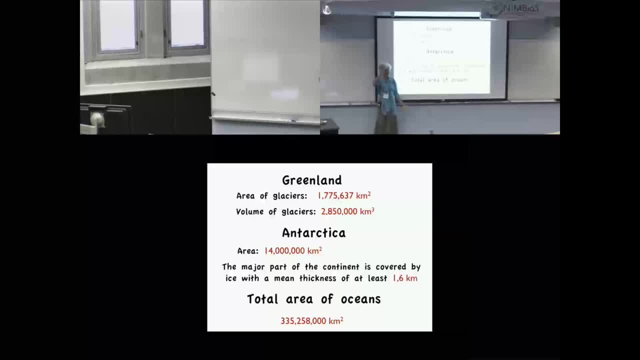 In Antarctica. I just found the area. The thickness is very high. I took a mean thickness on 1.6 kilometers, So 1,600 meters. That gives you a volume. Then you find on the internet the area of the oceans and you divide. 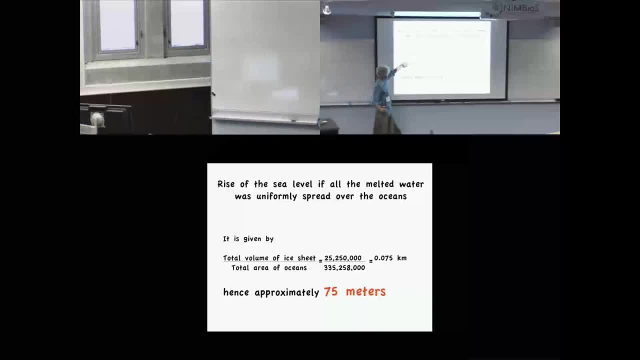 So the volume of the ice sheet divided by the area, you find approximately 75 meters. So when I first did that, I said, well, where is the mistake that I made? and then I went to internet and I found other people that had found the same thing and I discussed and there is no mistake. 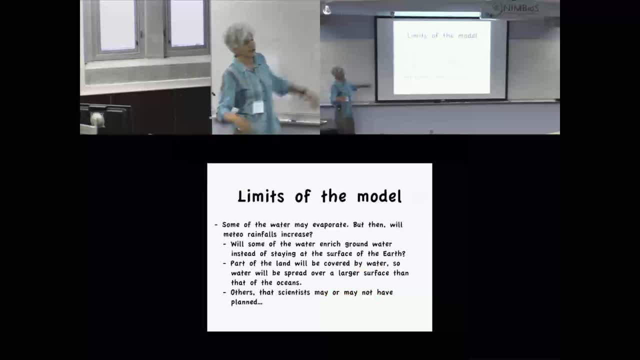 So then you can start the discussion in the classroom. What are the limits of the model? Well, maybe some of the water may evaporate, but then will it increase. the rain falls Maybe somehow good the water with and enriched the groundwater In the room. some people say that part of the water will go over the land, so that will be less over the ocean. 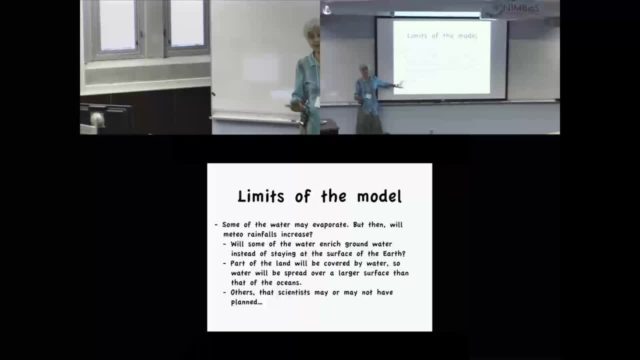 When we talk about something, what have we missed? It is one of the messages. We are thinking of some things, But we can make predictions with what we have thought of. but have we forgotten some important things? I will just discuss a little, for instance this part. 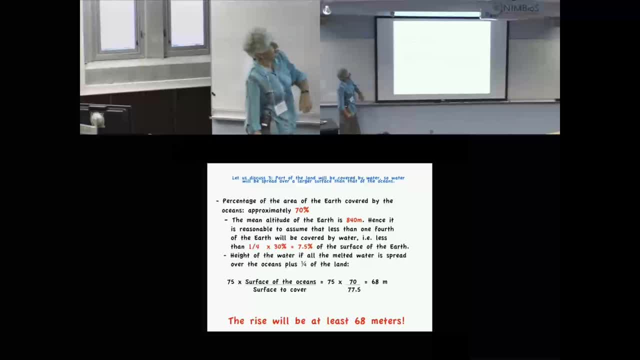 So well. the percentage of the area of earth that's covered by the ocean is approximately 70 percent. The mean altitude is 840 meters. That's all data you find on internet. So in the classroom you just go on internet and you just 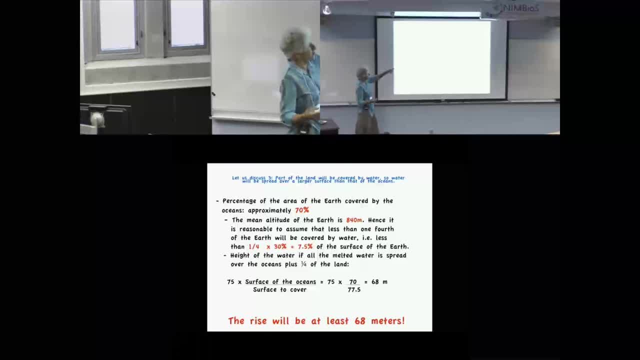 have the discussion with these things. So with this altitude, you could imagine that no more than one-fourth of 30 percent of the ground would be covered by water, So 75 percent of the surface of the whole earth, And then instead of 75 meters rise. 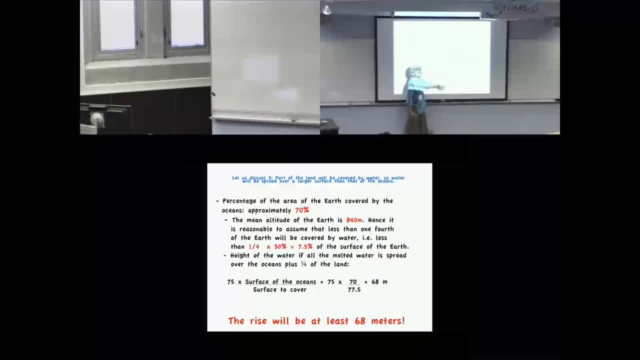 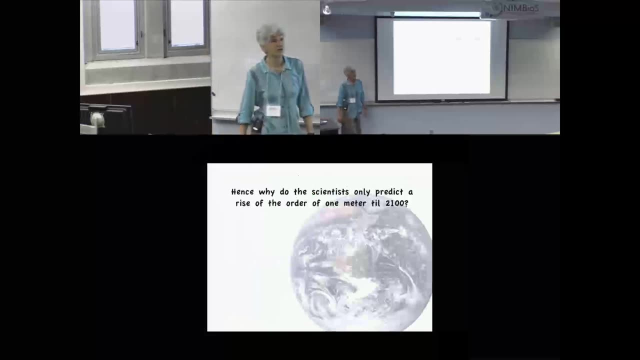 for 70 percent of the surface of the earth, you would go to 77.5 percent. Well, you just go down to 768 meters. So we have a big, big potential rise. Well, we hear on the news that the 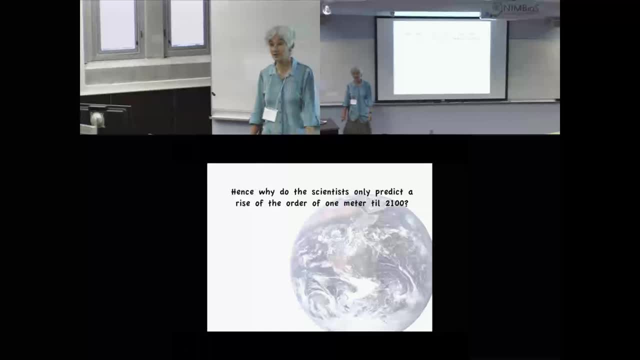 the rise would be of the order of one meter till 2,100.. So, in fact, I asked some Hervé Le Trut, some very well-known climate scientists in Paris, and he just told me: well, because the ice cannot melt so fast. 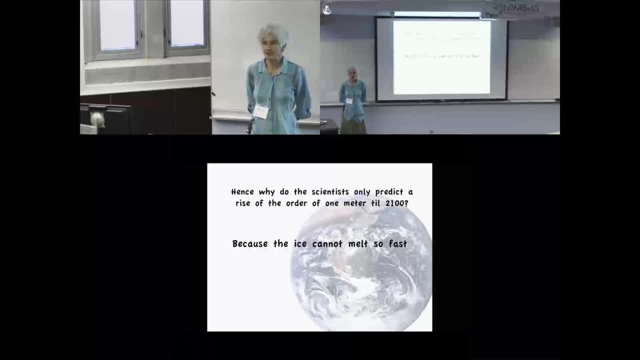 But you see that the official message is: they will just tell the rise by 2,100 will be of the order of one meter. So it's something that's hidden. They didn't tell us what's coming In fact, when we'll be by. 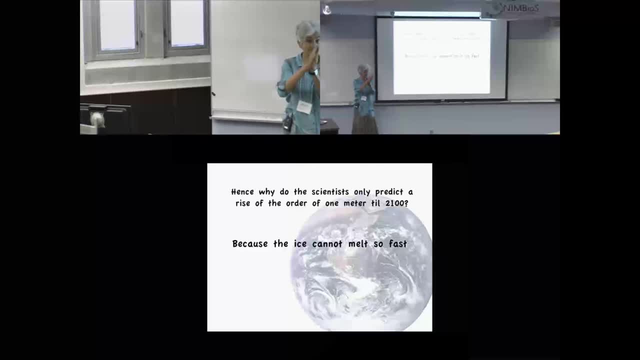 2,100, the steep will be stronger than now. So in fact, if you are to build your dams and things, you shouldn't build for one meter, You should build for much more. So we see that we must look beyond 2,100. And in fact, 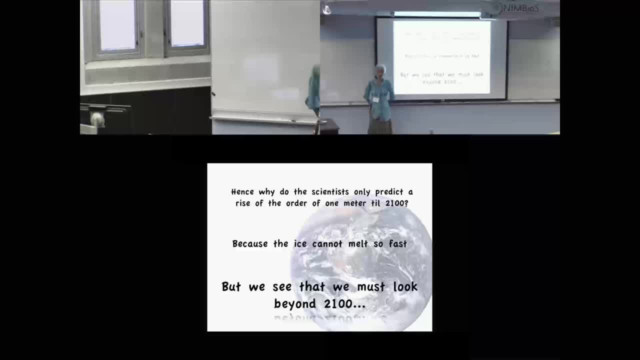 one question I will say: what haven't we put in the model? I was last September at the General Assembly of the International Council of Science in New Zealand. The International Council of Science is very concerned with climate change and all these things, So they work very. 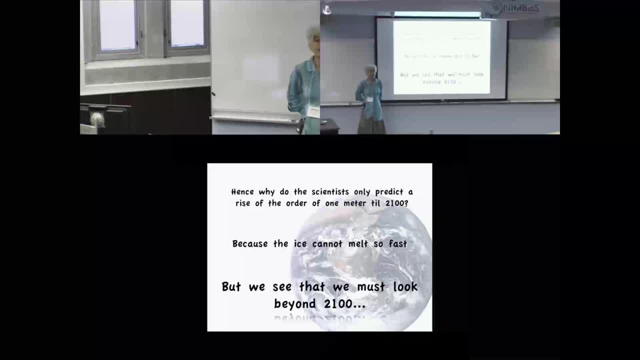 hard on this And there was a lecture that impressed me a lot from Butler- her name- about one new hypothesis is a potential collapse of the West Antarctica high sheet. So the ice is so sick in Antarctica that the level of the land is below seawater. 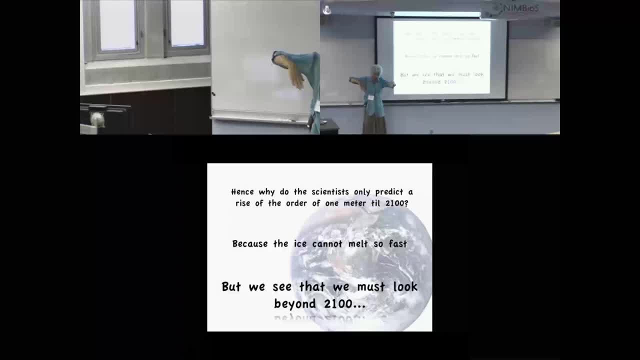 So you could imagine that you have seawater that could go underneath the ice and break some big parts, And if you have, once the ice is melting, it's like water on the ocean: it rises. So if the West Antarctica high sheet were to collapse- and this is a question mark- 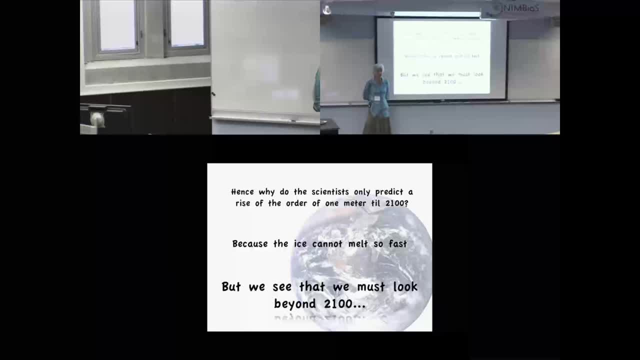 that would mean that could mean a rise of four to eight meters by 2,100.. So that's things we can Now I'm out of climate change. just a movement of tectonic plates, So they move on, viscous magma and 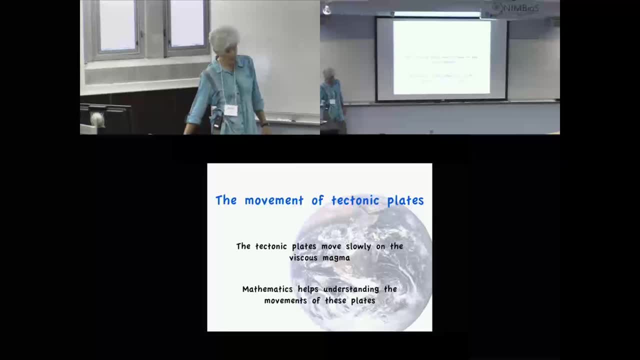 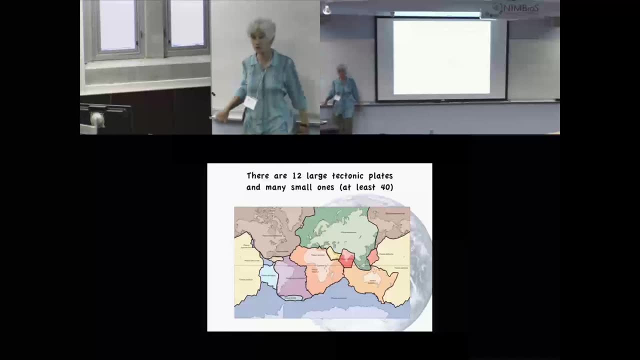 mathematics helps understanding their movement. So there are 12 big plates and now we're identifying new more, so more than 50. What's? I'm just interested to the mathematics behind. So how to describe the movement of a tectonic plate? Well, it's a solid. 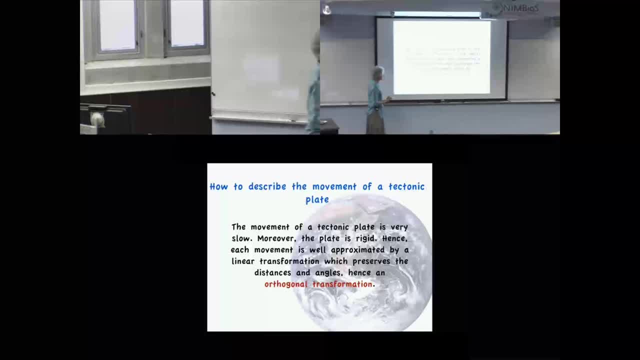 It's a solid on the sphere, So it's originally a rigid movement and then it's slow movement. So if it's a slow movement, a rigid movement of a sphere, then it's well approximated by a linear transformation which preserves distance and angle. So an orthogonal transformation And because it's close to the identity. 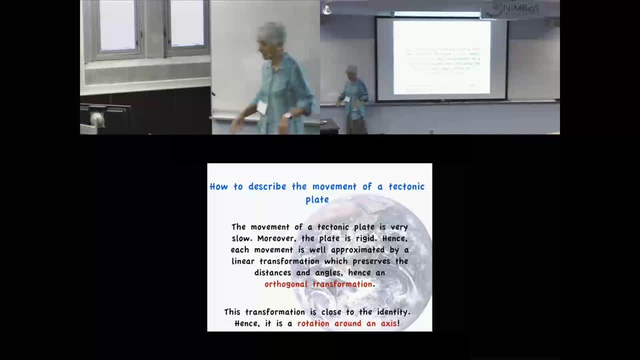 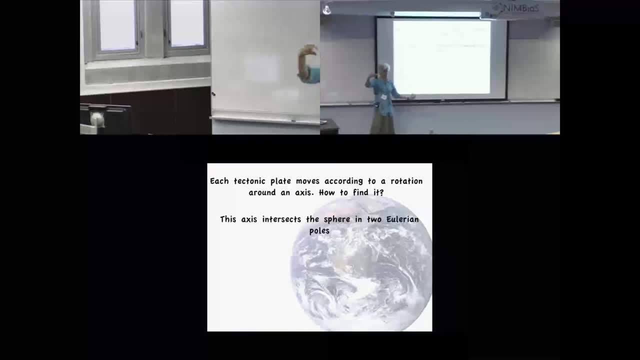 then it is a rotation around an axis, So the movement of. so if you want to describe a rotation, then you have to find its axis. So its axis would intersect the earth at two points and then you have an angular rotation. 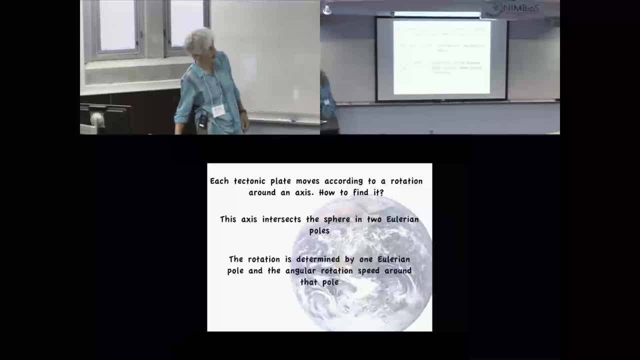 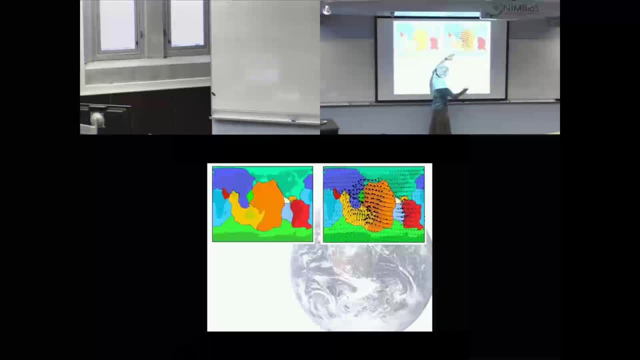 So you, so it's going to. so you see that you can the movement. well, what you have is here: you would have, for instance, the green, you would have an axis, and you have the rotation movement and that gives you the. 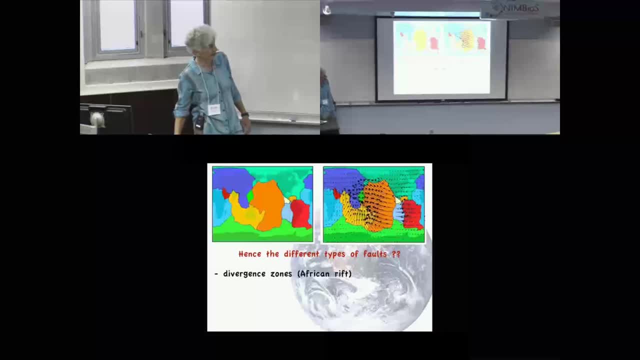 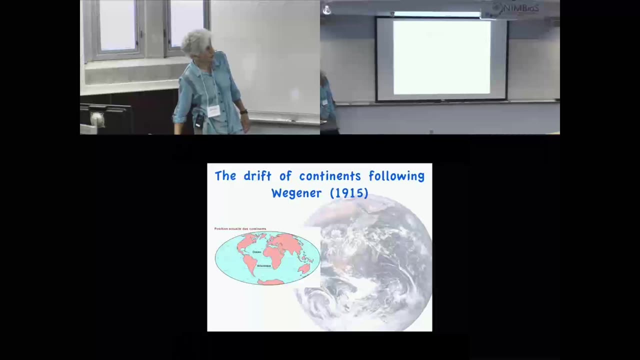 motion of the tectonic plates and that you can have the different types of faults, So divergence. when plates are moving apart, you can have convergence and you can have slides. It comes with the drift of continents. so the sorry, the slides. the images are in French, so 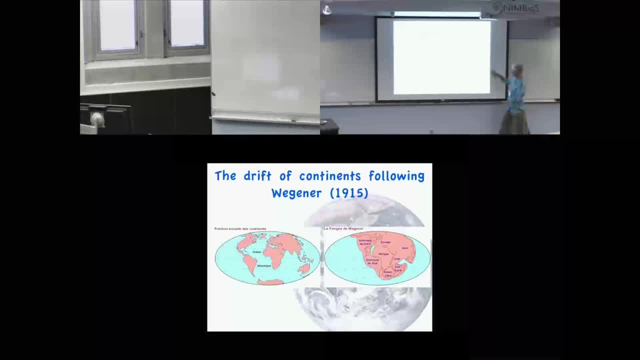 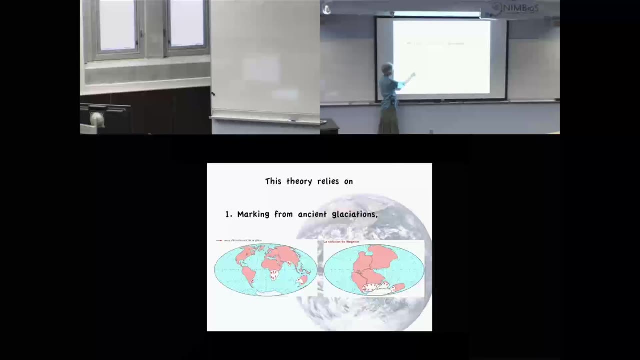 Wegener-Pangea. the hypothesis is that the continents were once all glued together. What's interesting is where the theory relies on, And then you have some marking from ancient glaciation. So why would the glaciation go like that? It's not natural that they would go. 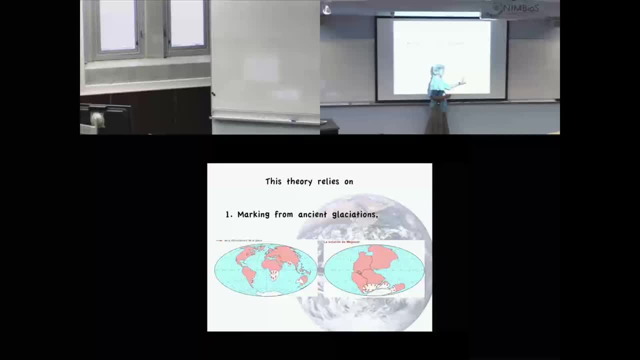 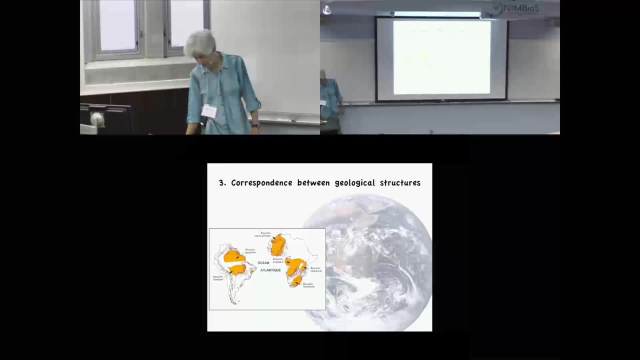 inland. Well, with the image of the Pangea then it becomes more natural. There are some similarities in fossils in regions that are far now from each other, and also correspondence between the geological structures. So now we have these geological structures. Look at: 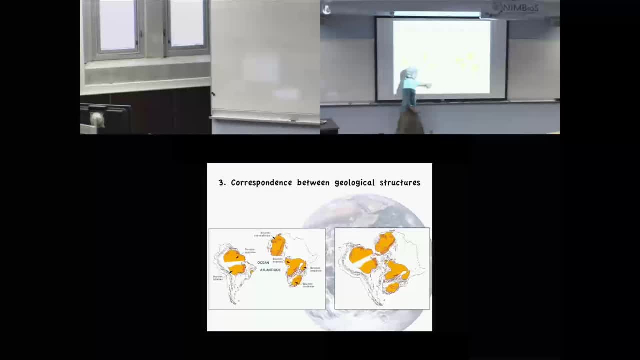 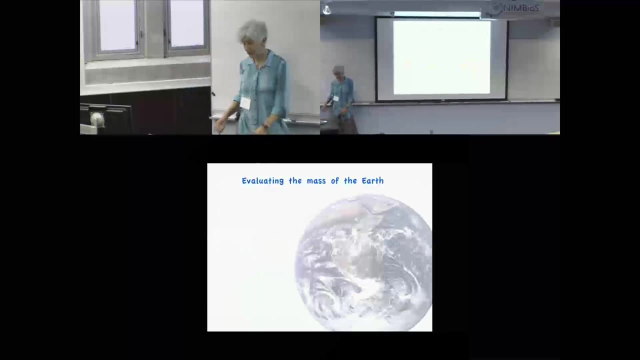 these two small pieces of mountains and when you draw the Pangea then they fit exactly like that. So I move from different questions. So evaluating the mass of the Earth. So you use Newton's gravitation laws and you deduce the mass. 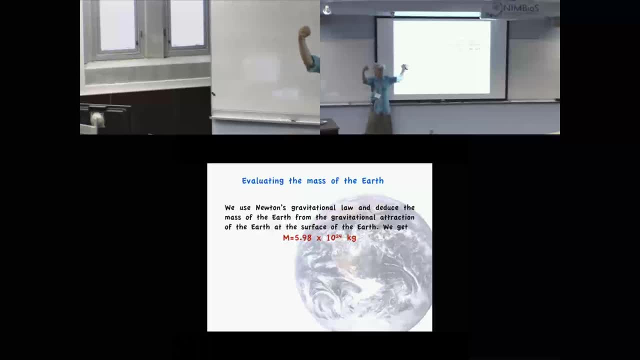 of the Earth from the gravitational attraction. You know that the attraction is the acceleration, 9.8 meter by second square, and you know the universal constant. so you find the mass of the Earth. You know the density near the surface: It's between 2.2 and. 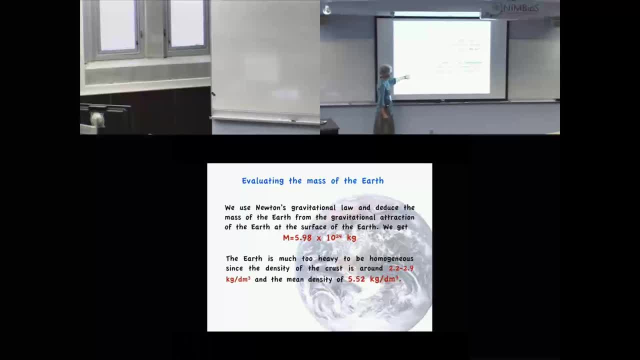 and 2.9 kilogram by decimeter cubes, And you calculate the main density from the volume, which is 5.52.. So that means that what that tells us is that the interior of the Earth is much heavier than what we observe at the surface. 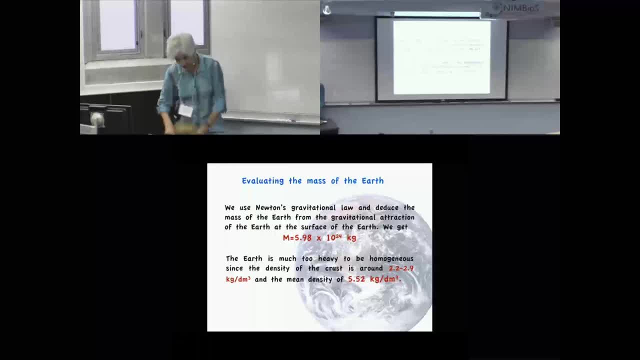 When I have this kind of problems and I go to the public I say, okay, that's like I don't see what's inside the Earth. But then what I do is that I put my mathematical glasses and then I understand I can see inside. 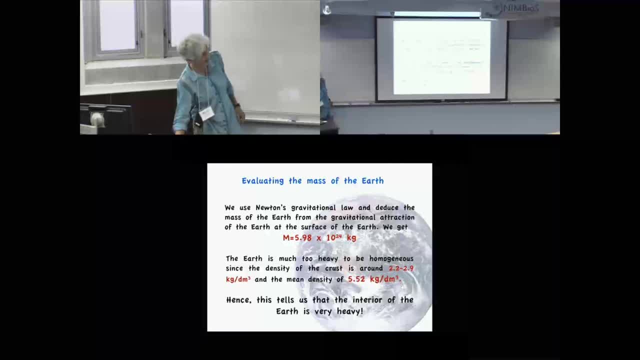 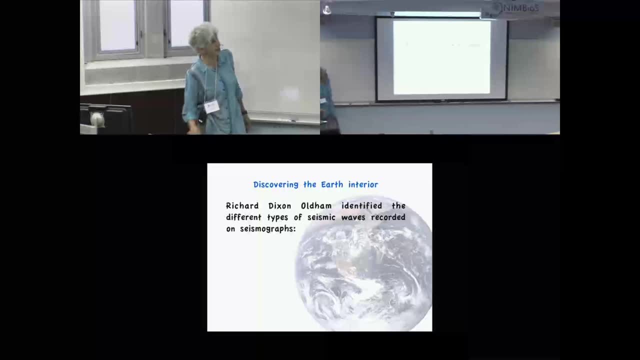 then the Earth is very heavy. So it tells us that the interior of the Earth is very heavy. So, in fact, putting our mathematical glasses, this is used to discover the Earth's interior. So when you want to discover the Earth's interior, 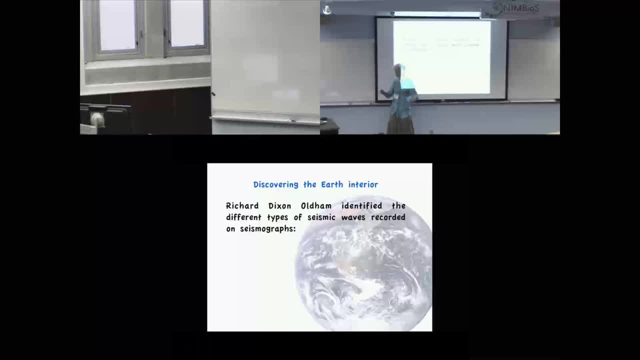 you just study the seismic waves and what they tell you on the surface. So you have two kinds of waves. You have the pressure waves that travels through the viscous interior and you have the shear waves that are damped in the mantle, and then you don't record them. far from the epicenter. 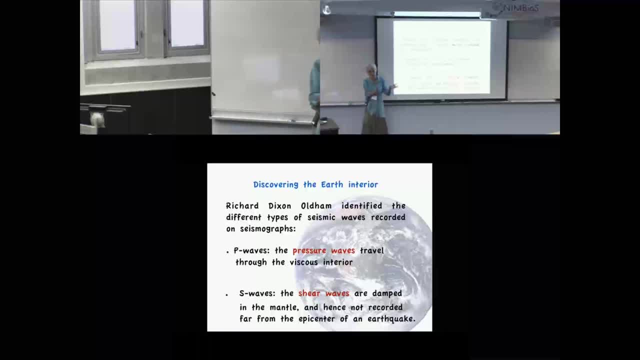 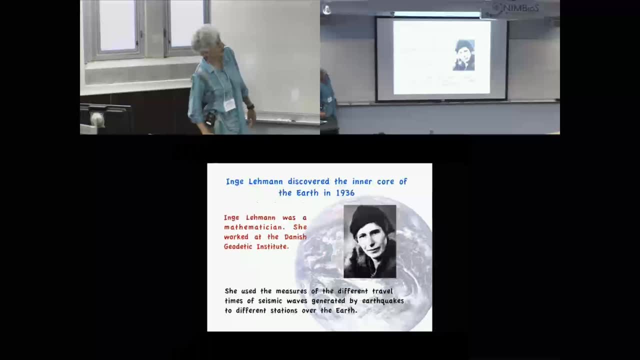 of an earthquake. So that tells you that in fact the interior is viscous, because otherwise you would register the shear waves very far from the epicenter. So, going further, in fact, for the people who want the details, I have written an article. 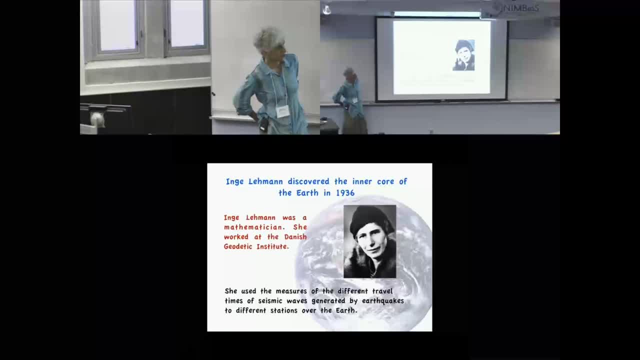 in the college mathematics journal of the MA. So Inge Lehmann would use the seismic waves to discover the inner core of the Earth. So it's interesting as a story because she's a woman mathematician And so it's a discovery she made in 1936.. 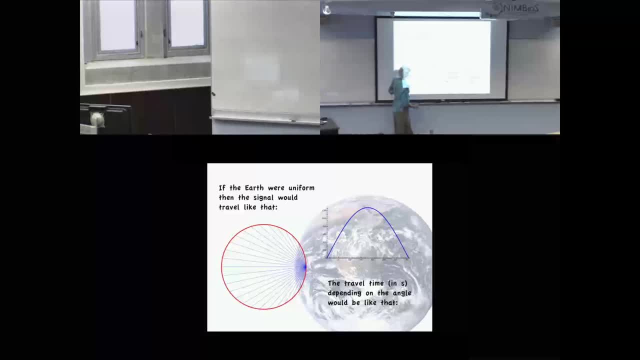 So if you have- suppose you have an earthquake here and you have- if the Earth were uniform then the waves would travel like that, And then you will record them at different stations And then you know. okay, suppose you know the time. 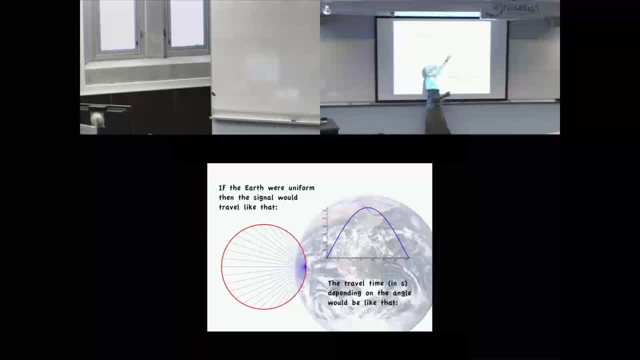 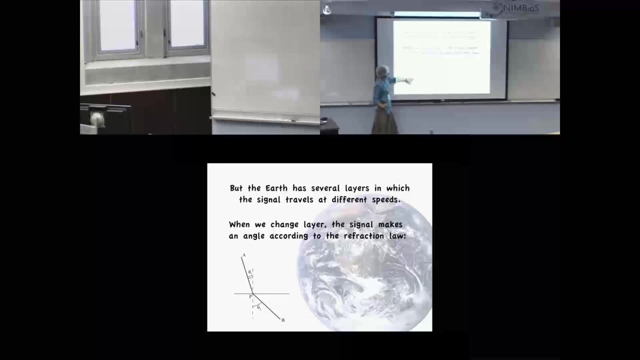 then you can measure the travel time. So you get a travel time like that, depending of the angle where you are. But it's known that the Earth has several layers And when we change layer, well the signal would make an angle according to the refraction law. 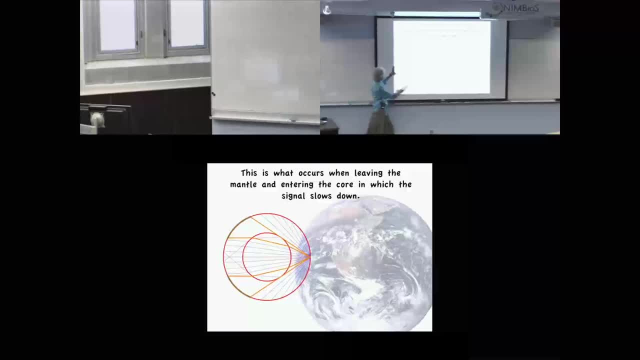 So this is what occurs. So when you have the mantle- so this is the baby model from Inge Lehmann. So she took a speed of 10 kilometer by second in the mantle, And then you enter the core and you go, you slow down to eight kilometers. 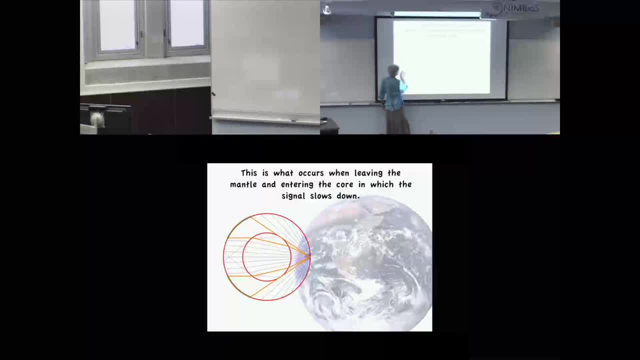 And then so the waves are bent like that. What you see is that, in fact, because of this, so you have the tangential one, and then in these regions you should record no signal. So no signals are detected. So in her tall model, between the angles, 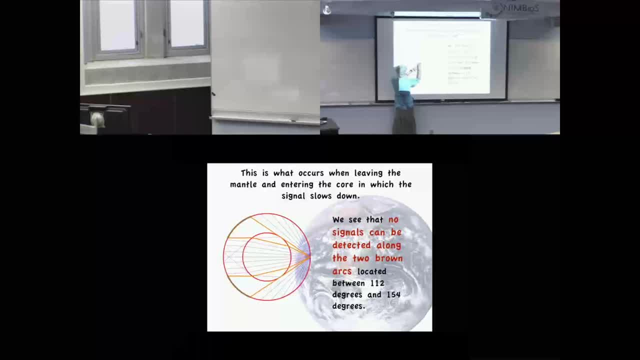 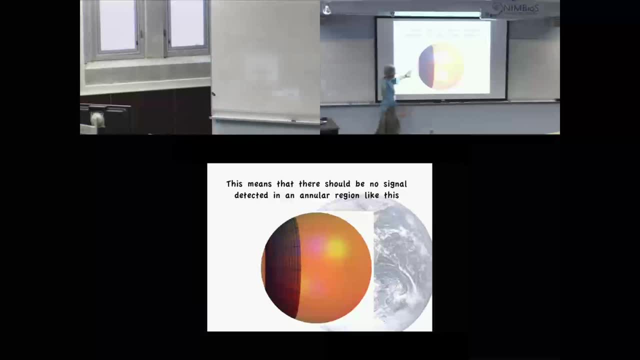 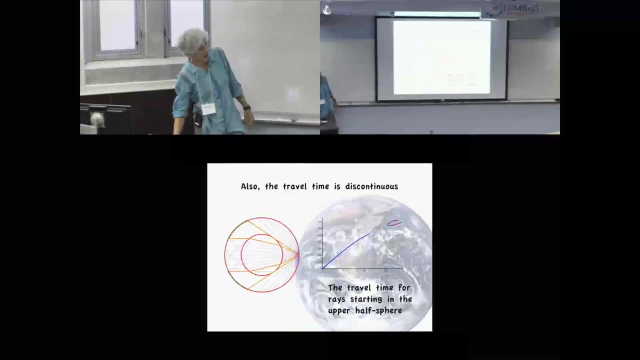 so from the center. so 112 to 154 degrees. So that means that from your epicenter you have an annular region where you should record no signal. Also, the signal, the travel time is discontinuous. You see, for instance, here you can have some signal. 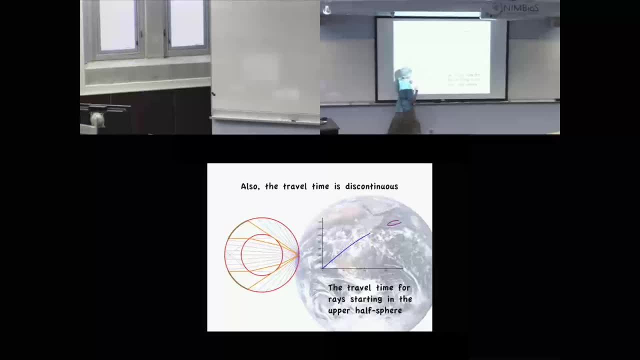 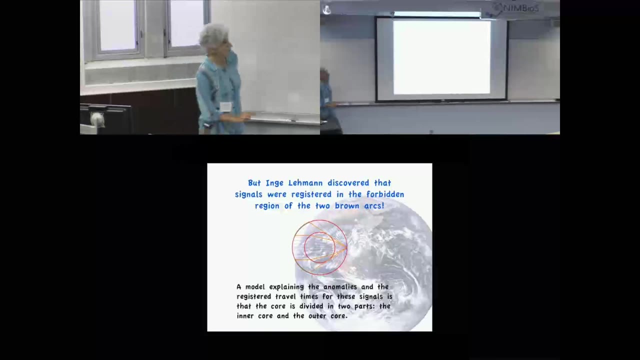 like that, but you can record another one that would be refracted. So this is why we could have signals are arriving at two different time. But then she discovered that there were signals registered in the four billion regions, And then what she did was to 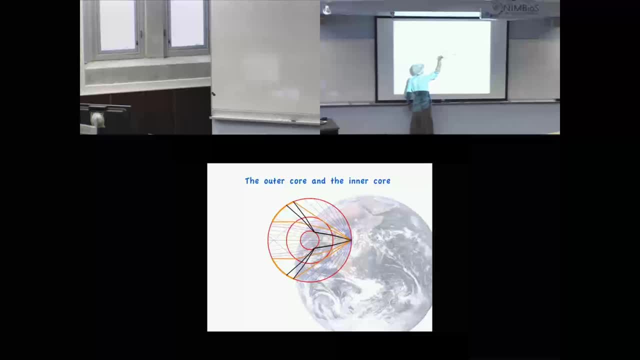 she had an inner core here and in the inner core the signal travels faster. If it travels faster, then if you arrive with an angle, you are going out, And if you arrive quite tangentially, then you will be reflected. And because of this inner core, 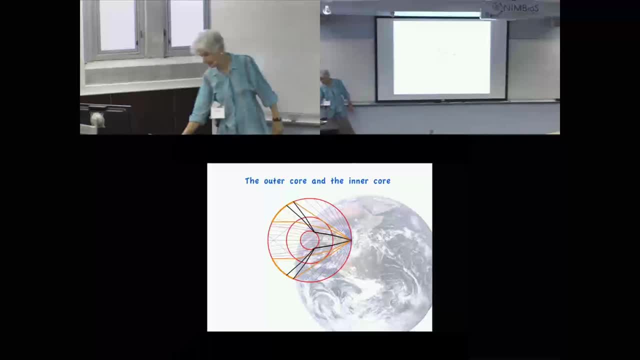 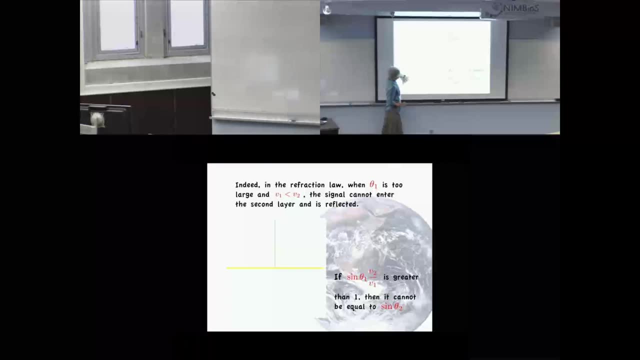 then you could register some signals in the forbidden region, So in fact in the refraction law. so I will just have an animation. So if you arrive so here you are slower and you go to faster, So when you have it tells you that in the second region. 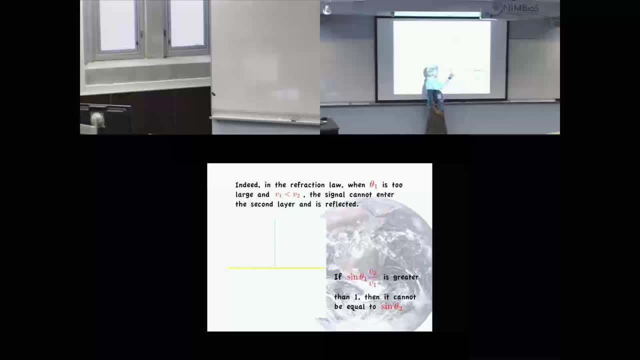 you should have the sinus of theta two, which is equal to this quantity. But if this quantity is greater than one, then you have no solution And then the signal is reflected. So, as you see, the material when we discuss this example, 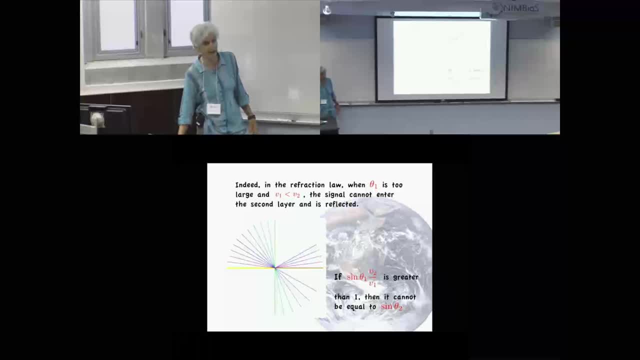 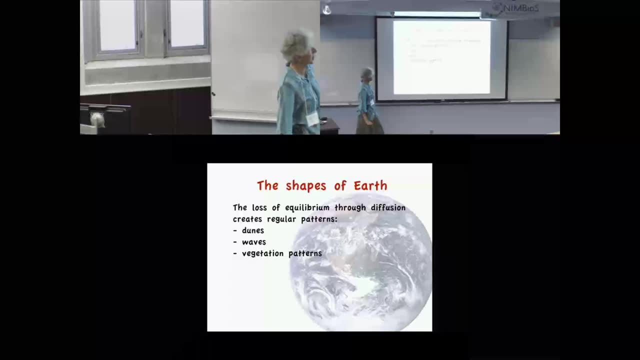 then we are working around reflection and refraction- I'm changing subject- So the shapes of earth, So it's the loss of stability. Suppose you have a flat land with sand, So it's very, very flat, And then you have this flat land with sand. 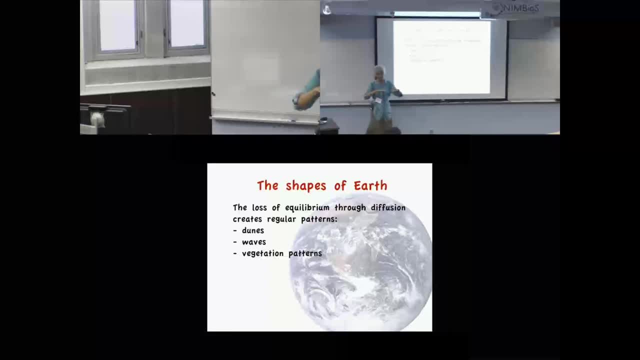 And then you have the wind that starts blowing. Well, you have it with snow also And then. so then you may have a small irregularity and then it starts growing because it stops the sand. So, in fact, when you will always have wind at some time, 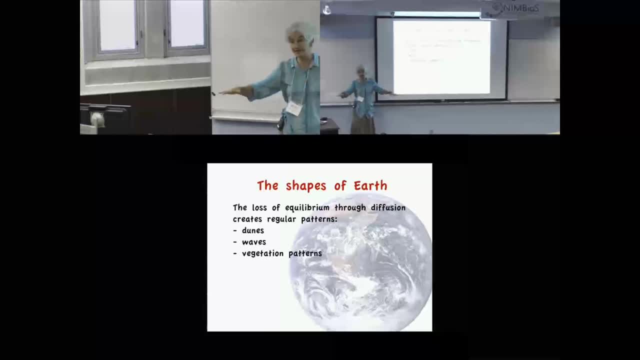 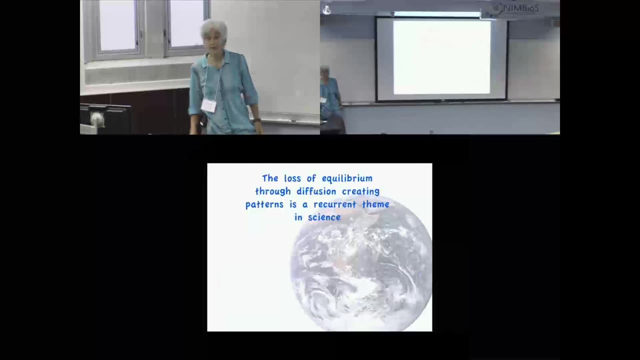 So on earth you never observed some flat area of sand, and you will. it will create regular patterns, So dunes, waves, vegetation patterns, so So it's a very it's a recurrent theme in science, So it's a very important this idea of Turing occurs. 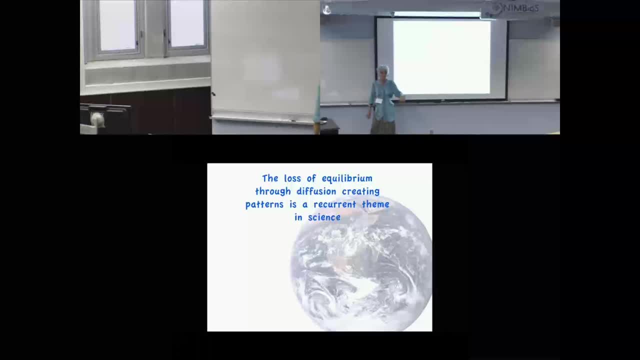 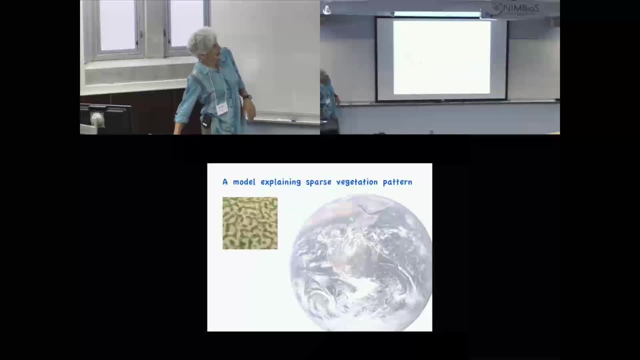 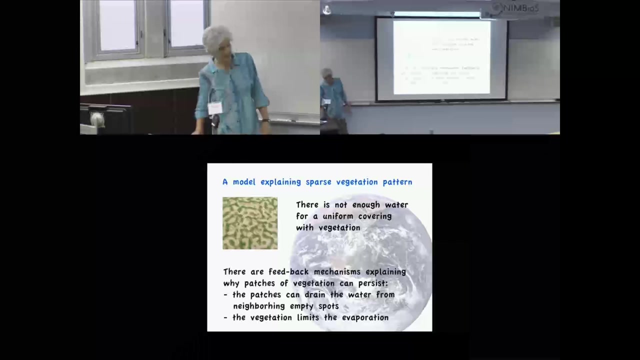 in many, many areas of science. In fact, it was his hypothesis for morphogenesis. So this is why it's important, So it's nice to introduce the idea because it's so general and unifying in science. So let's talk about the 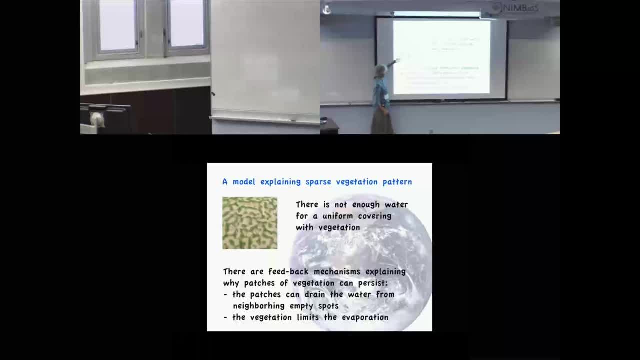 All that would explain the sparse vegetation pattern here. So you have- you don't have enough water for uniform covering with vegetation, And then you have some feedback mechanisms. So in fact, when you have some small patches, well, they can drain the water that. 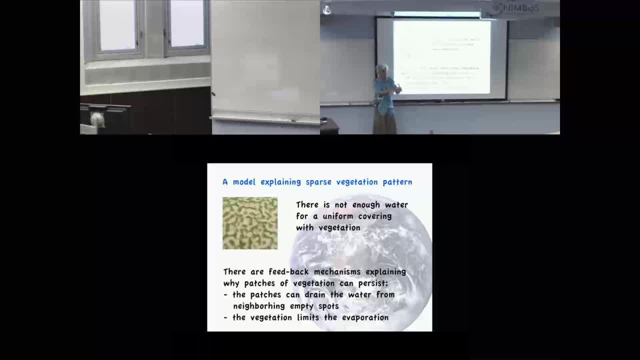 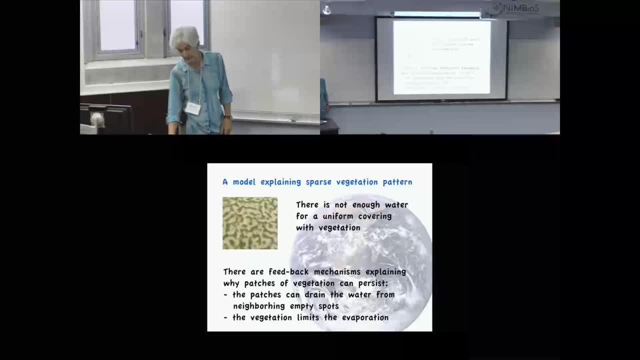 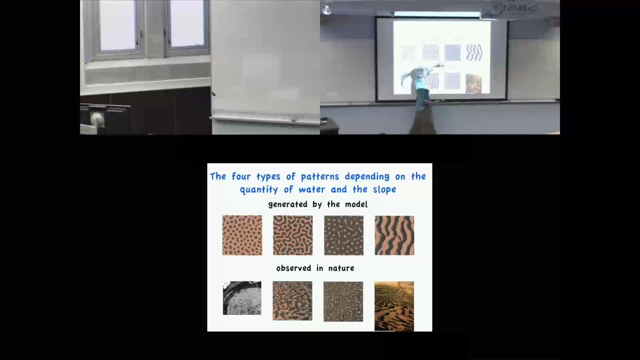 the evaporation, so it will stay. when you have a little water, it will stay more humid. So the model gives, predict, generates some patterns, so you could have spots, labyrinths, gaps and you could have stripes. Well, these patterns are exactly observed in that nature: the spots, the labyrinths, the gaps and the. 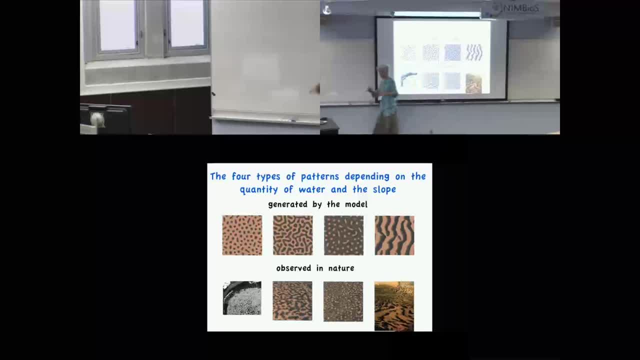 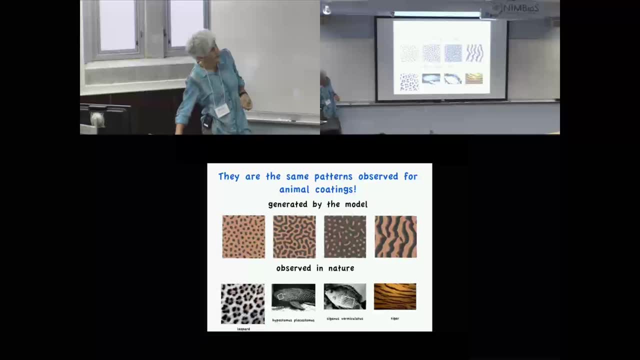 stripes. you have them on slopes, So you get what's very interesting where just you want to attract the public. it's that the same model works for the patterns observed in animal coatings, And then you have the spots. so this I found on internet. so don't look at the, but you have the labyrinths, you have the gaps. 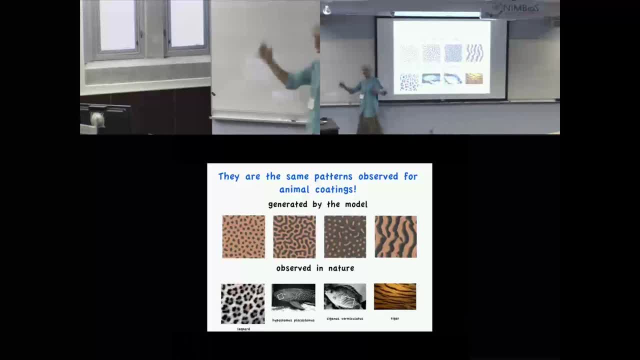 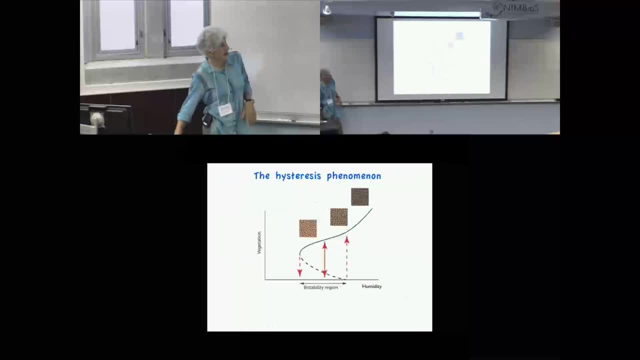 and you could have the stripes, So you have, I think, a great idea to present the labyrinths, the gaps, and you could have the stripes, So you have. I think the great idea to present is the unifying idea In our vegetation. so we observed the high terraces. 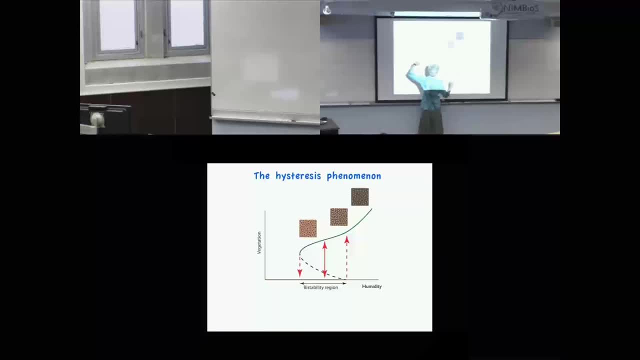 phenomena. so you have humidity, you have vegetation, and then you can have, in this region, bi-stability, so you can have either an equilibrium with no vegetation at all, or you can have the gaps, the labyrinths, and if you have more humidity you have the 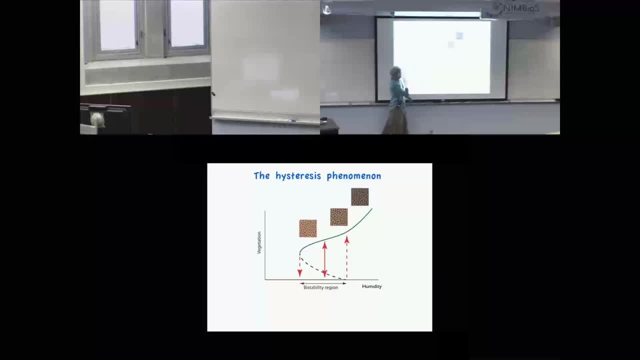 sorry, the spots, the labyrinths and the gaps. The lesson from this graphic is suppose, for some period, the humidity, you have a drought period, so then you lose your vegetation, it dies, so you come back here and then you can when the next. 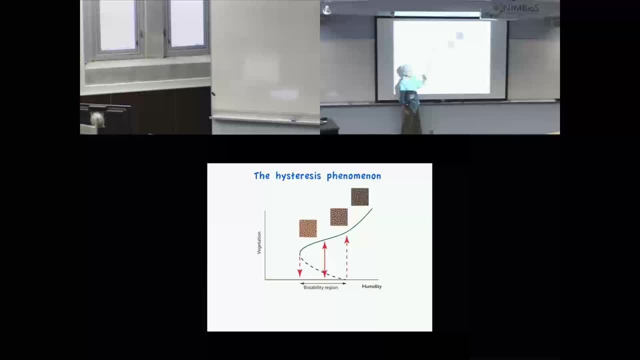 year, the humidity comes back, the vegetation doesn't come back. You need to go very, very far to be able to come back. So a very important idea which is very general. so we have passed a tipping point. no return is possible and the idea of a tipping point is again a very unifying 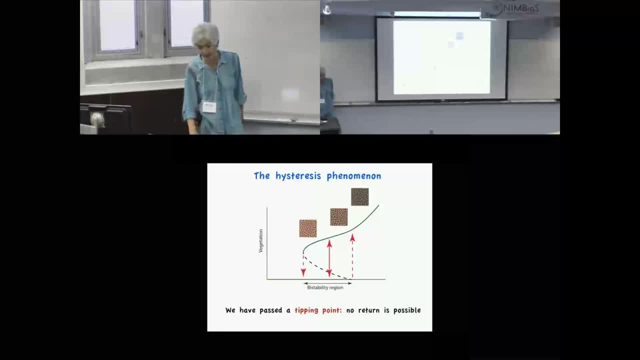 idea when we present some modeling, When I was preparing public lectures about mathematics of planet Earth. so there were the four teams and one team was a biologically diverse planet. and then I was saying, okay, what I wanted, just one element for the public to present and was wondering: okay, so you? 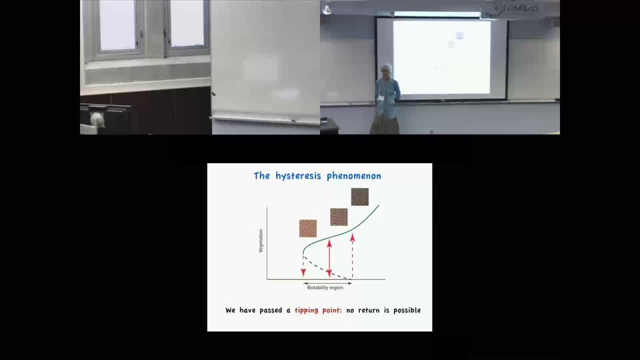 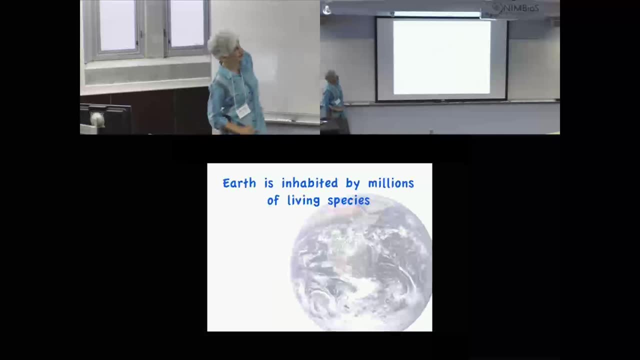 know, And so then I discussed with some biology, and this is the team that I liked and that I choose for the lecture. So Earth is inhabited by millions of living species, and then where does all this biodiversity come from? So, just understanding the mechanism that produces the 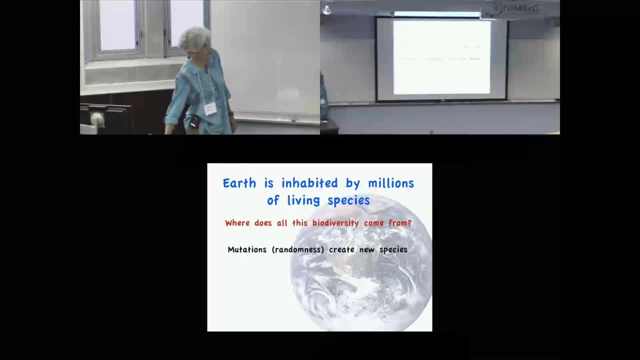 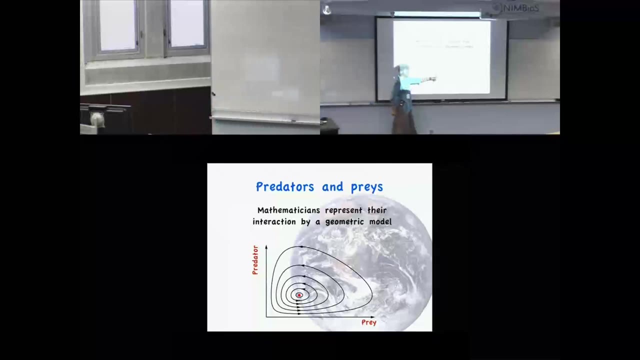 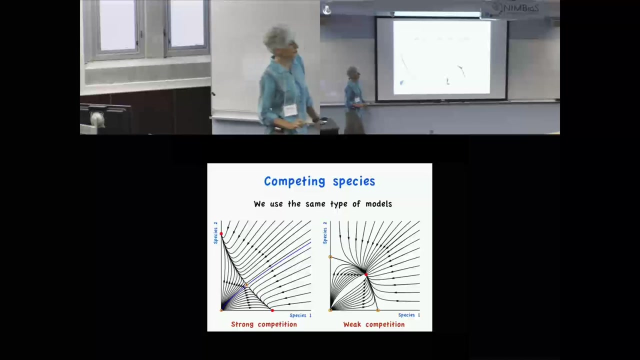 biodiversity. So of course you have mutations, randomness create new species and then these species interact to survive. So when we present modeling, we present small models, predator and prey, so we can have cycles of probably- you know, I don't go into the details- We can have competing species, so we can have 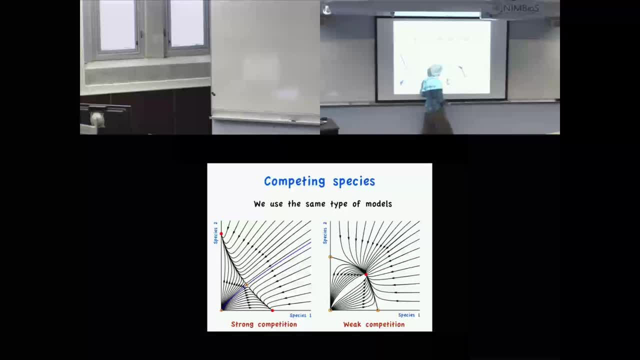 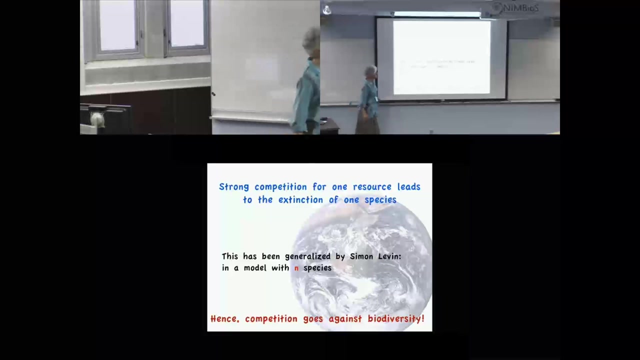 aably into theunuz数, But I want say that those are particular. So in weak competition we can have that two species survive, but in strong competition we see that there is frontier and on one side species two win and on the other side species one win. So in fact the lesson from this is that 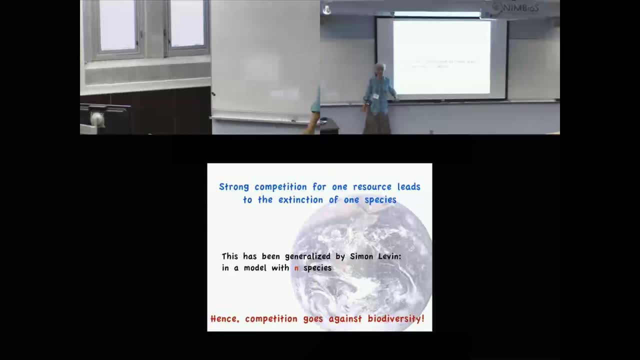 strong competition for planet resources leads to the extinction of one species- and this has been generalised by Simon Levinavantz- of one species, and this has been generalised by Simon Levin. So the lesson is that competition provides a sense of Seit. Five Reasons during competition is that competition for man resources leads to the extinction of man species, And that is what several бокs are all divided into other��가es. This might be even exploratory. 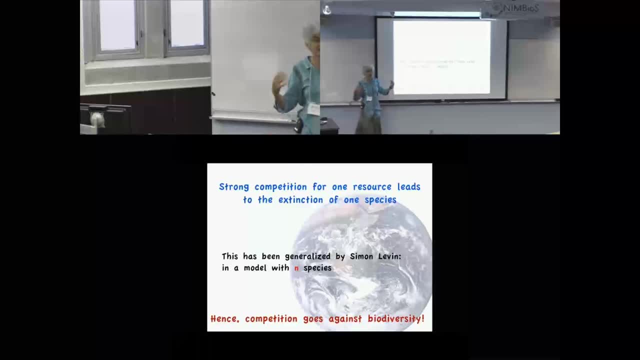 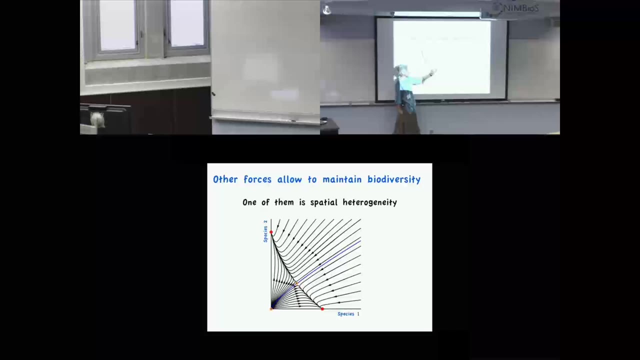 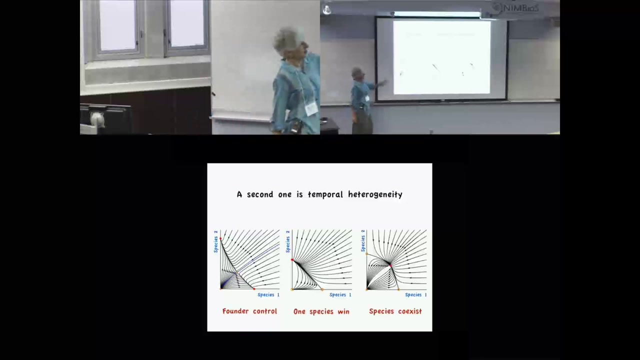 goes against biodiversity. That means if the question is what maintains biodiversity, we should understand it. There are other forces. One is spatial heterogeneity, where you may not have the same initial conditions in different places of the planet. Another one is temporal heterogeneity. Well, the conditions are not always the same. You can have one species that's favored by winter, another one that will be more prosperous in the summer, and one that will suffer from the drought, another one that will suffer from too much humidity. So, because of the changing of conditions, 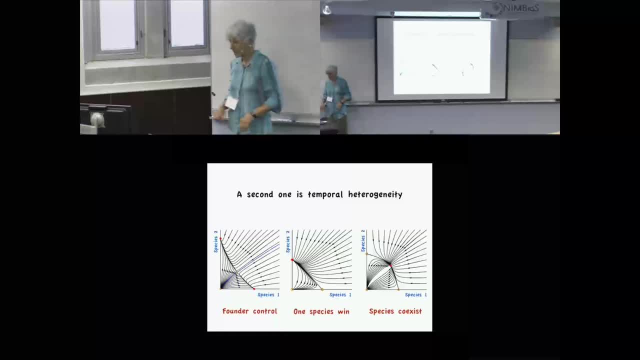 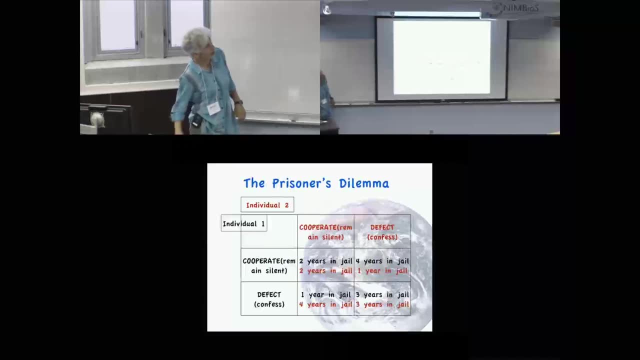 this allows. But the very important force also that was introduced was cooperation. So that's illustrated by the prisoner's dilemma. So I'm individual1, and you are individual2.. We have two choices. We can choose to cooperate or to remain silent. 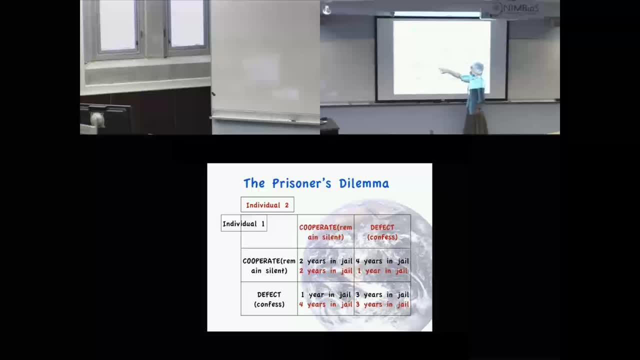 Suppose you choose to cooperate: If I cooperate, I get two years in jail. If I defect, I get one year in prison. you're in jail. Suppose you choose to defect: If I cooperate, I get four years in jail. If I defect, I get three years in jail. So, whatever you do, my best choice. 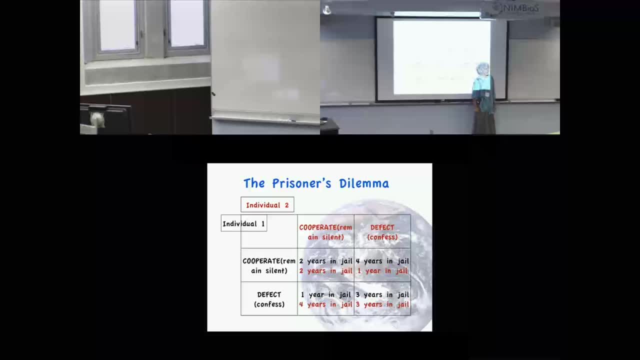 is to defect, Okay, but maybe you will make the same reasoning that I did, So maybe you will choose also to defect. So then we will both defect. then we will both get three years in jail. Maybe we should have cooperated. So in fact, that's. 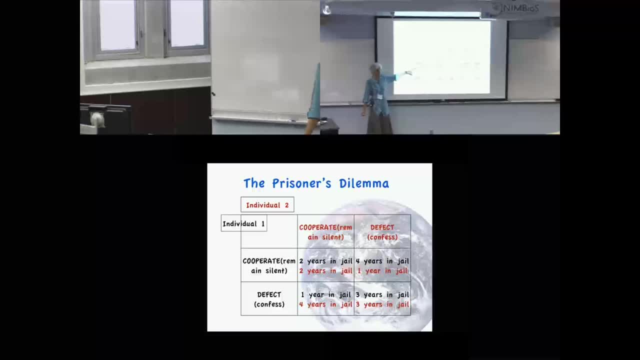 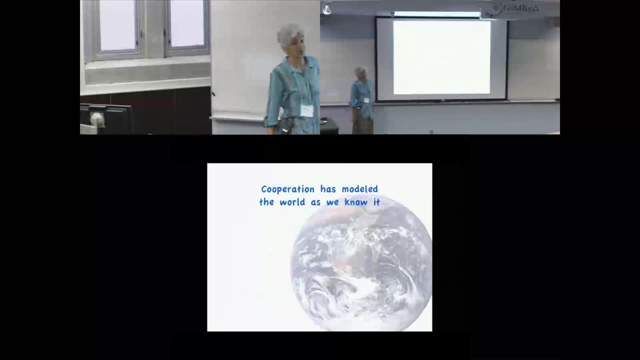 well, that's the kind of things the nations are facing with the climate conference next December in Paris. This is well-illustrated So I won't go into the details because time is passing, but Martin Nowak has really observed five mechanisms in the world that makes. that means that the 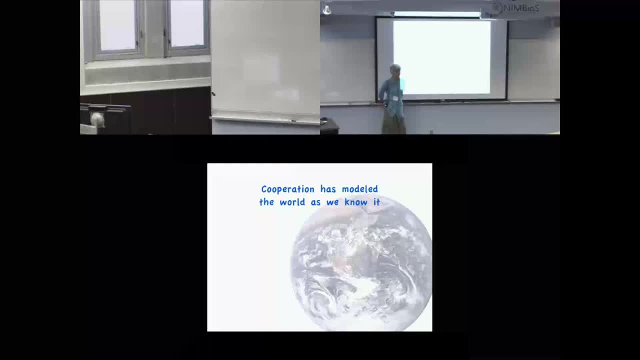 natural species do in fact, cooperate, and this is important for biodiversity. The lesson is that cooperation has modeled the world as we know it, so it explains the preservation of biodiversity, and it's everywhere present in the human organization of the planet. I'm almost out of my time, so I won't explain the next. 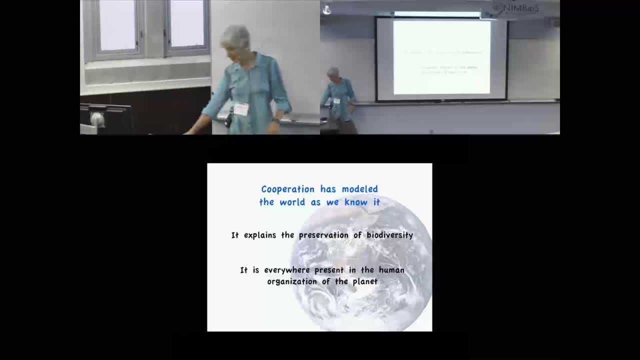 slides but just say the title. Now I go on many things. so the Greek that could see that could measure that the earth was a planet. So I will go on many things. so the Greek that could see that could measure that the earth was a. 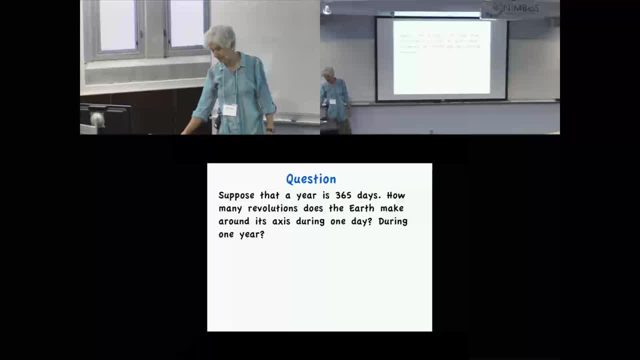 round and the size. Funny question. so how many turns does the earth do during one year around the Sun? Well, during one day you need to make one turn around your axis, but then a little more because you move here. So you make 366 turns. 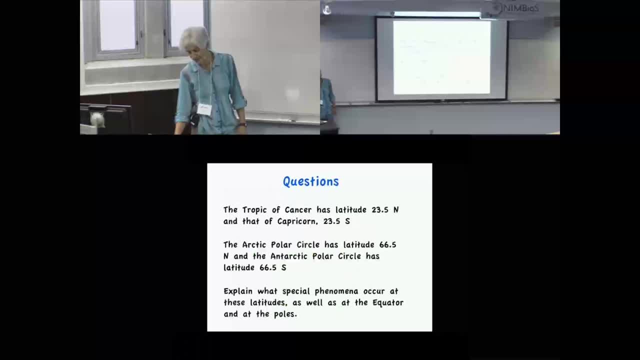 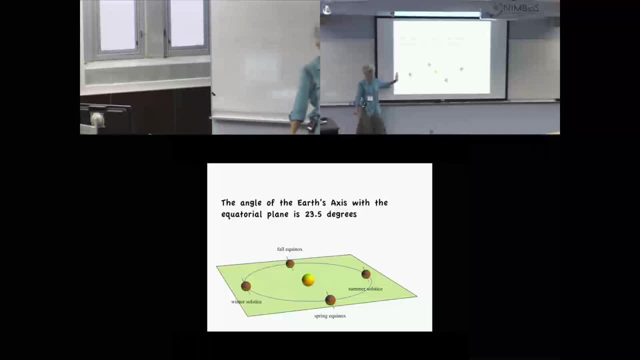 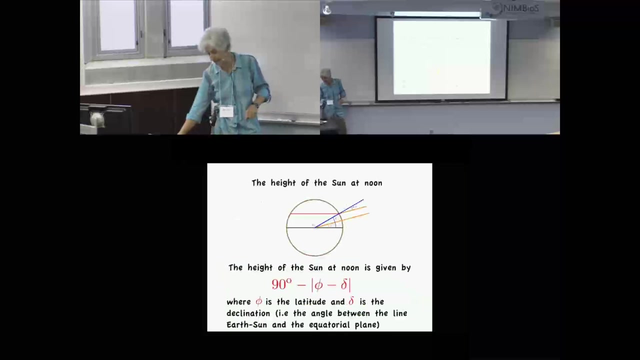 during 365 days. Mechanism of the season. so that's, most students in school don't know that the mechanism of the season is because the axis of the earth is slanted. so in fact we, just when we do this in our mathematics course, we just fill the gaps in their culture. the 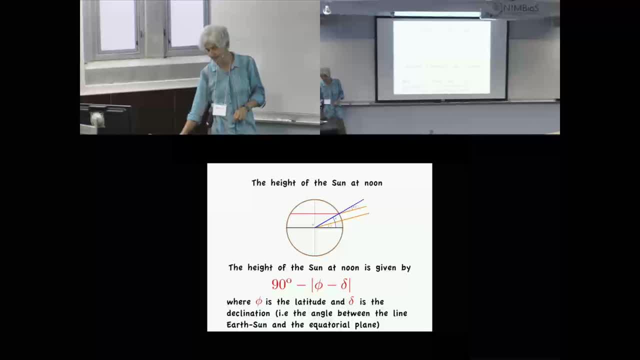 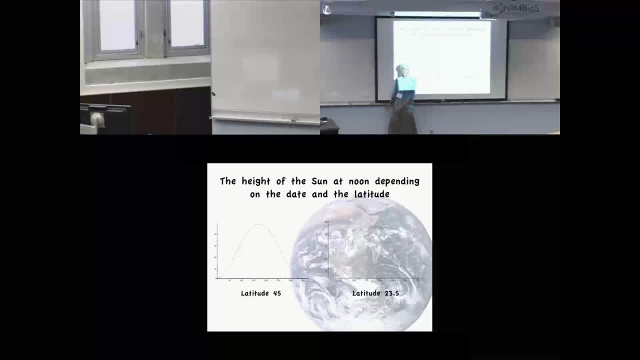 height of the Sun at noon, depending on the latitude and the season. so of course you wouldn't be surprised that at your latitude the curve is like that. what is interesting is to have the curve when you are between the tropics and then you see that, for instance, at the equator. so you have two maximum and with a sharp slope, so these curves are interesting. the equation of time: have you already noticed that in the northern hemisphere the sunset is sooner on December 10 and on December 21?? so 21st is the shortest day, but the sunset is later on December 21st than on. 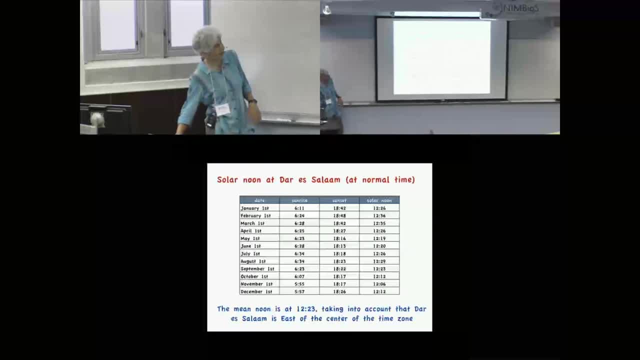 December 10. so this comes from the fact. it's called the equation of time. well, here I have the data for Dar es Salaam. when you look to the solar noon, well, the time changes by an order of 13 minutes during a year. so it's a mathematical. 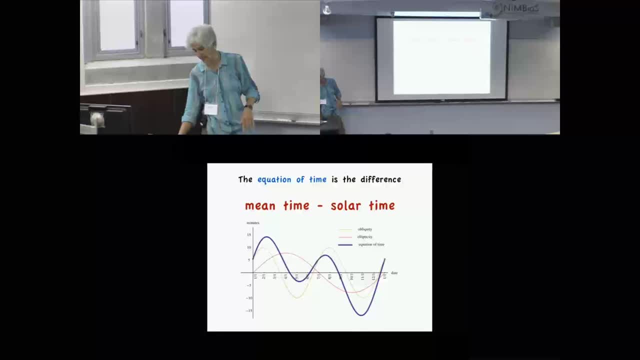 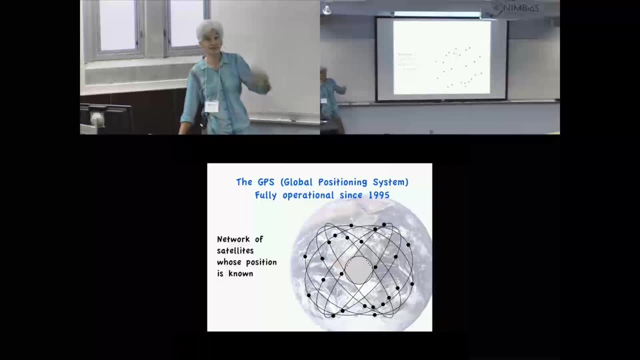 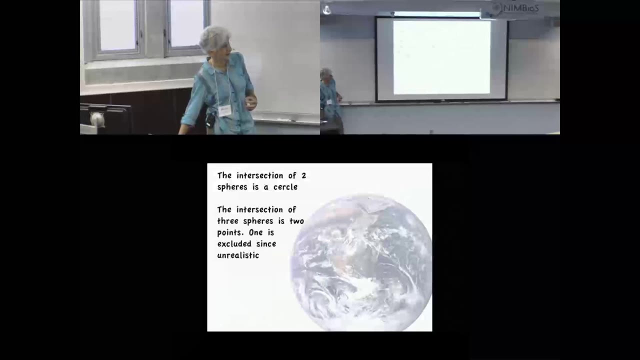 problem to give an explanation for that, but I don't have time gps, so how does it work? so it's: what is your distance from a satellite? and when you have this, then you can calculate where you are. so you are at a given distance from a satellite. so you on this sphere, given distance from this. 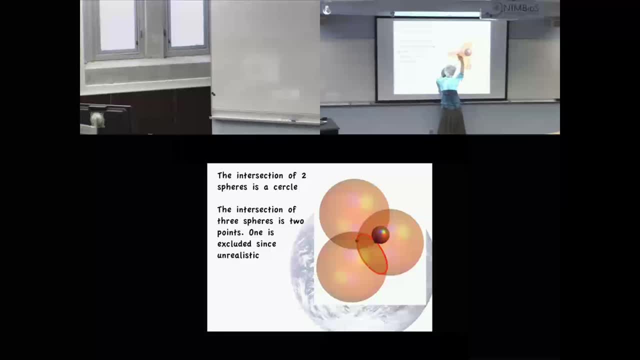 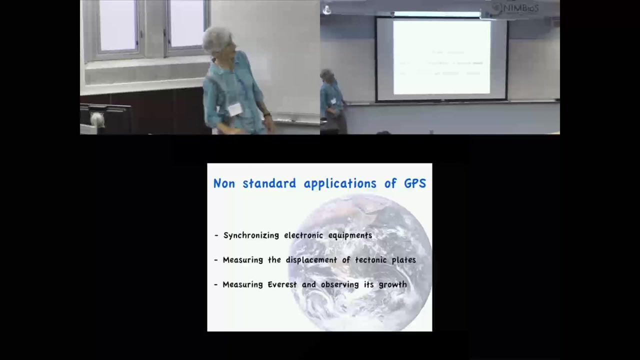 satellite. so you are on this sphere. the two spheres intersect on a circle. you are the different distance from this satellite, so you are on this sphere which intersects in two points, and then you choose the point that's close to Earth- Some non-standard applications, so it's used to synchronize electronic. 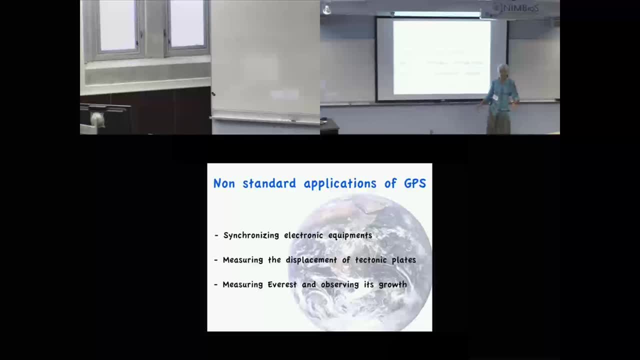 equipment because in fact you need more than three satellites. you need four, because the clock of your GPS is not the same as the clock of the satellite. so your receiver calculates the shift between its clock and the clock of the satellite, and when it has done this, you can use it to synchronize. 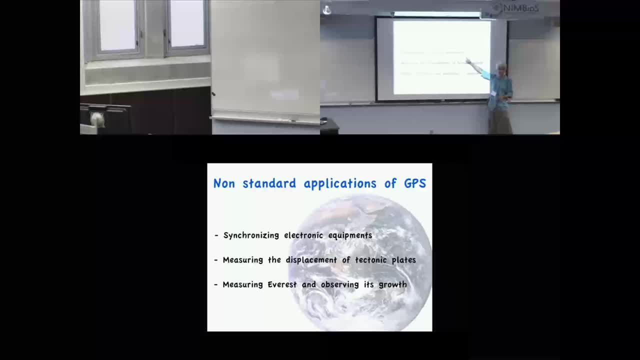 electronic equipment. All the electric grids are synchronized by GPS, which are much cheaper than atomic clocks. That's how you measure the displacement of tectonic plates and you measure the growth of mountains. Maybe I should stop here, Okay, well, how you give definition. What means altitude? 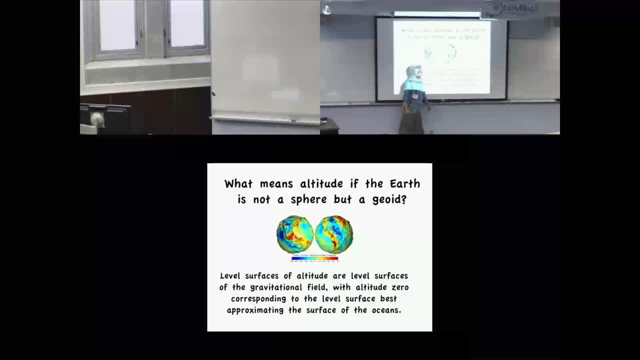 if the earth is not a sphere but a geoid. So altitude? so in fact you use altitude, well, some constant altitude, it's a level surface of the gravitational field. and then for altitude zero you choose the level surface that best approximates the surface of the ocean. So that gives the 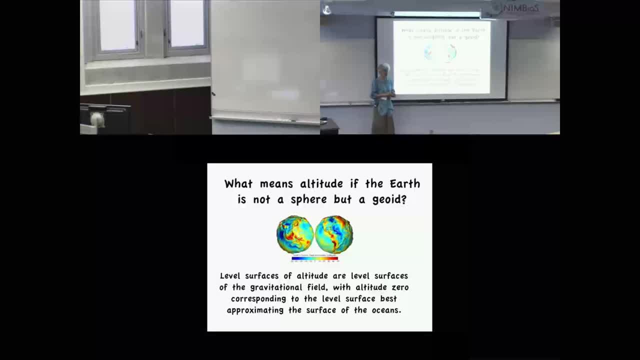 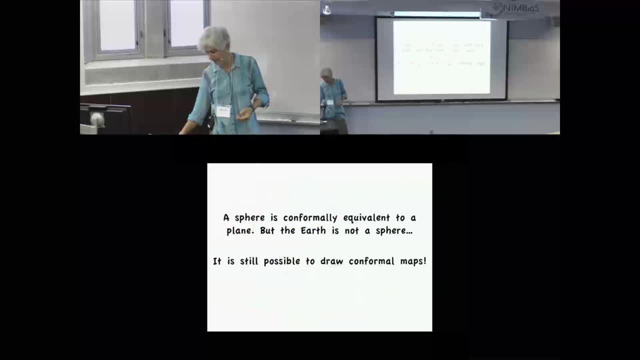 role of mathematics, on how you give definitions in some other scientific disciplines. Then I have other things in cartography, so how you make maps. but I will stop here and we'll have more time to discuss other ideas during the workshop. Suzanne, are these slides going to be available to us so that we can put it on the website, please? 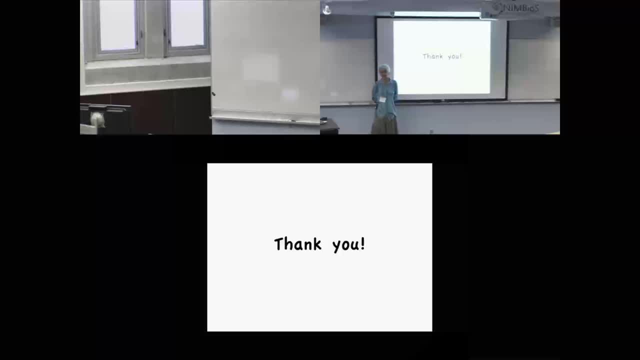 Of course I will. Anyone else Yes. So how did your students that you presented the first example with the 75 meters? how did the students respond when the 75 meters first came up? Were they shocked? Did they have any idea how high 75 meters are? 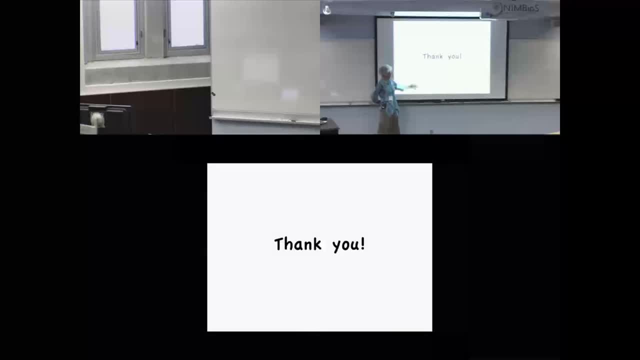 This one. I haven't done with the students Several of the things that it's because I teach a course- mathematics and technology- and the students have to do projects And And then I would so, for instance, the projects with the season, with the equation of time. 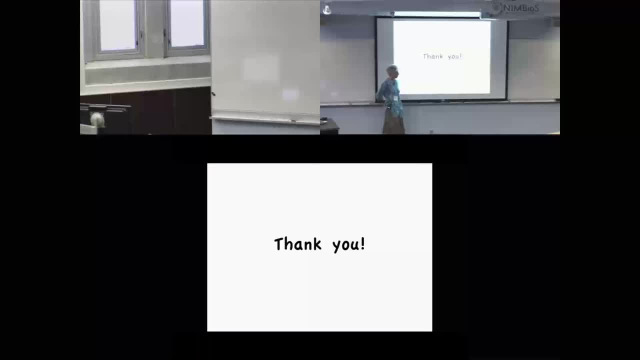 why it's not noon always. these are parts of the projects that I. the projects could be on technology, but I found that all these things are interesting projects. I could say the rise of 75 meters. I had done it when I was. 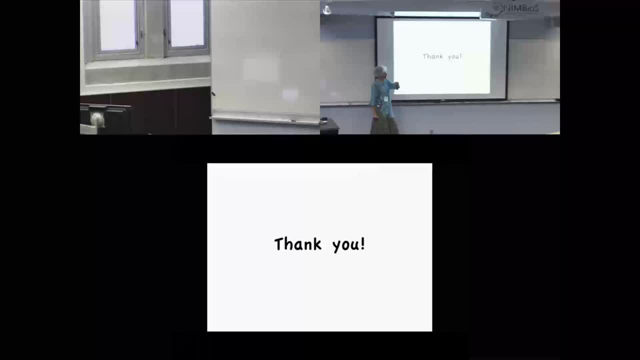 while we were having this competition and I was just- and I put it on the blog of MP but it could get unnoticed with some, but I found that well, for me it's striking that we never, never hear, we just hear the rise will be well, it used to be half a meter before 2100,. 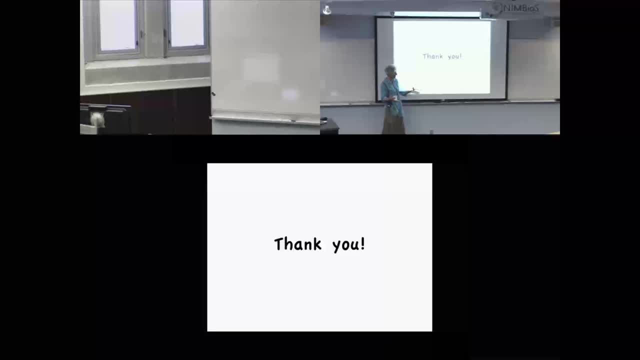 now it's between half a meter and one meter. In fact, NASA last week or recently said it will be of the order of one meter, but we never, never hear of what could come afterwards and what's the potential threats, which is something, I think, which is a very important message. 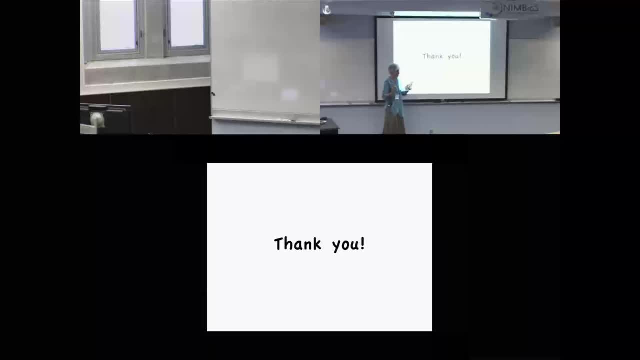 And as I tell that there are, because that's the problem we have as mathematicians we give, we study models, but the model only contains what we put in it, And that's where- and that's where it's also a danger, I could say, because we put some varnish on science- that 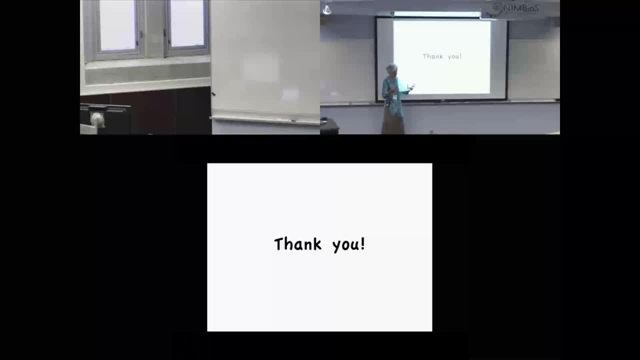 and then? so we have a responsibility, because we can't say what the model will produce, And this is where we can not work alone. We have to work with other disciplines. What do we put? what do we put in our models? Have we forgotten something essential?